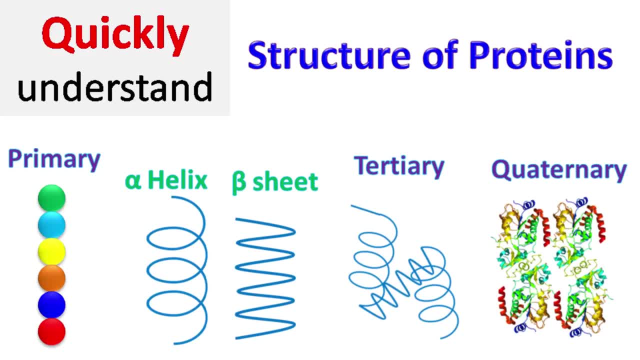 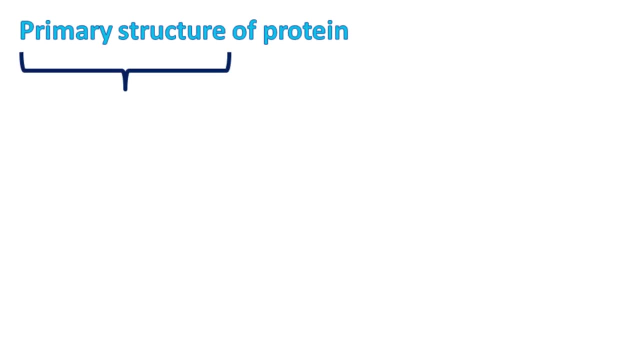 Hey everyone, Quickback Chemistry Basics. here Let's talk about structure of protein. So the proteins have a primary, secondary, tertiary and a quaternary structure. Let's talk about each of them. Primary structure of protein. Primary structure of protein is a linear sequence. 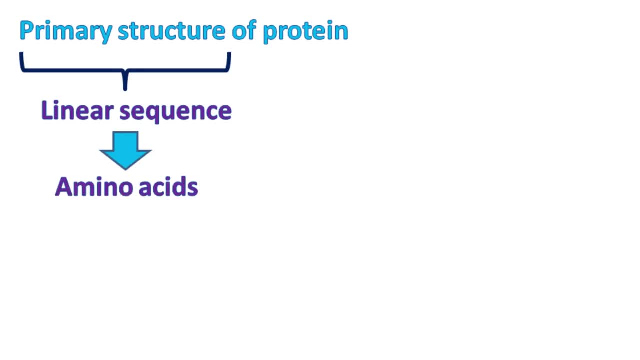 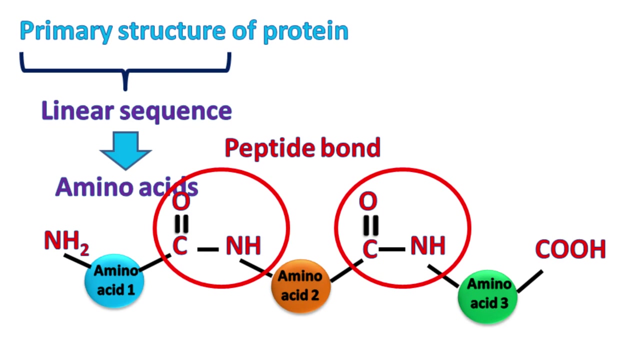 of amino acids present in the protein. This linear sequence of amino acid is either written in a three-letter or a one-letter form. Now these amino acids are attached with each other by a peptide bond. Now the primary structure of protein is always written from the N-terminal. 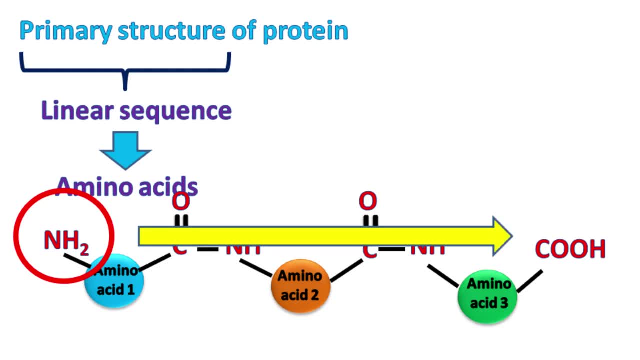 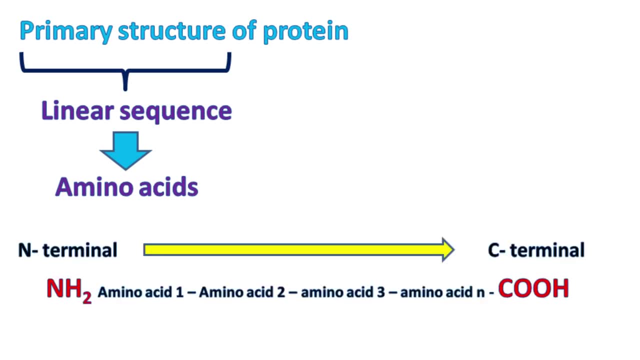 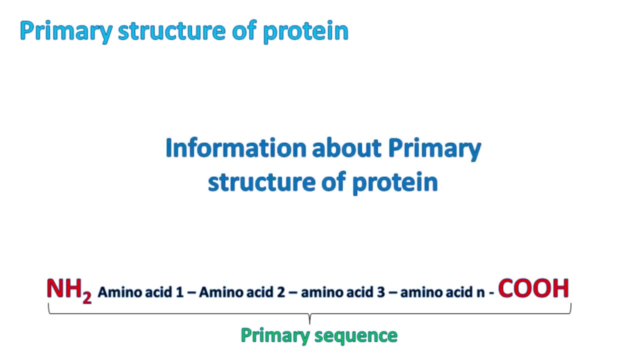 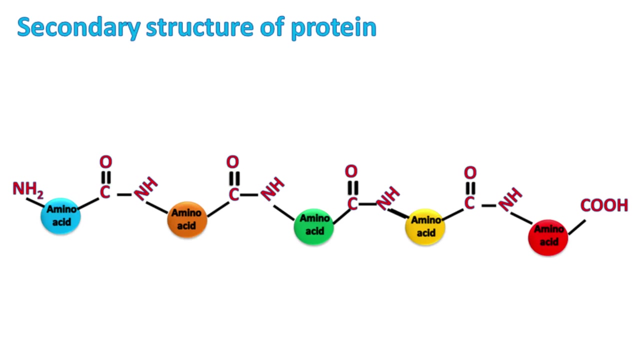 of the first amino acid to the C-terminal of the last amino acid. The information of the primary structure of protein can be obtained by sequencing the gene that encodes the protein. This information can also be obtained by sequencing the protein itself. Secondary structure of protein: Now in the primary structure of protein. 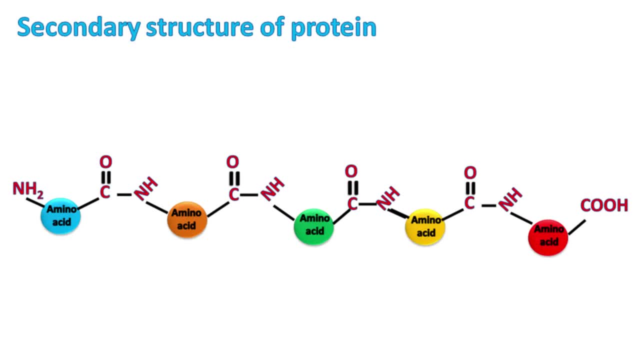 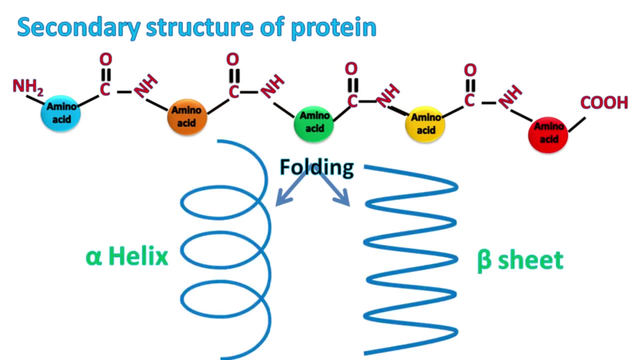 the amino acids are linked by a peptide bond and the peptide bond has an attached with the carbon and the nitrogen attached with the hydrogen. Both oxygen and hydrogen have the ability to form hydrogen bond and this results in folding of the peptide chain either in alpha helix or the beta sheet. 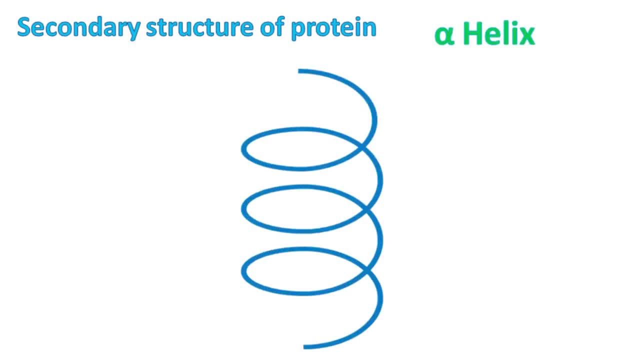 Let's talk about alpha helix. Alpha helix is the most common secondary structure of protein. In the structure, the protein attains a spiral shape, such that the side chain of amino acid remains outwards. The alpha helix is stabilized by hydrogen bonding. This hydrogen bonding is formed between the hydrogen 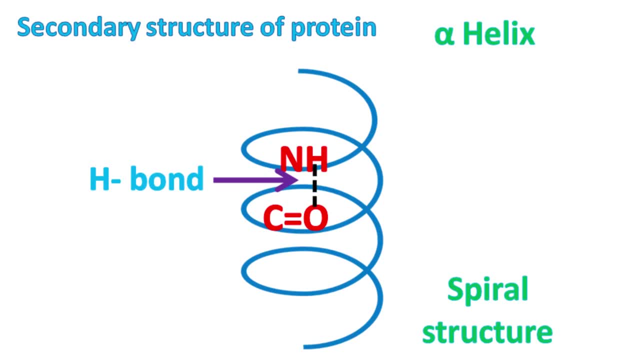 of nitrogen and the oxygen attached with the carbon. Individual hydrogen bonding are of course weak, but collectively they are strong enough to stabilize the spiral structure. All the proteins in alpha helix form a spiral structure. No peptide bond except the first and the last participate in the hydrogen bonding.